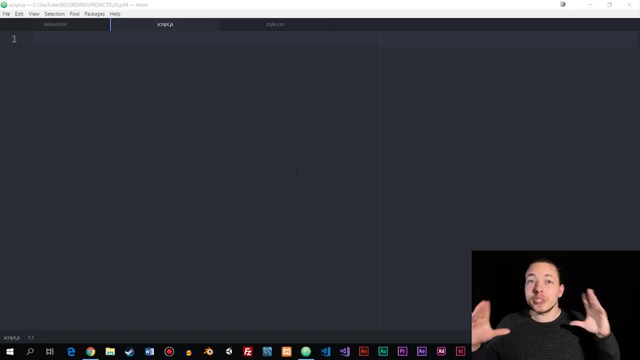 Today I'm going to teach you about events inside JavaScript, And events is a huge feature when it comes to using JavaScript, And events is something that happens all the time, anytime we use a browser or anytime we use a website. For example, if I were to resize the browser, if I were to go, 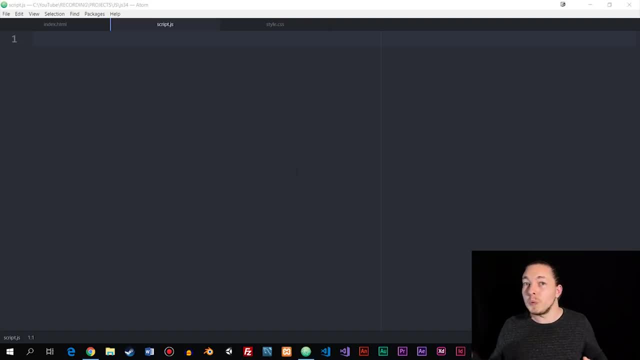 to another website if I were to click a link inside a website, if I were to move my mouse around inside a website, if I were to scroll. anytime we do anything inside a browser or inside a website, we call it an event. Now, the first thing you should know about events is that we 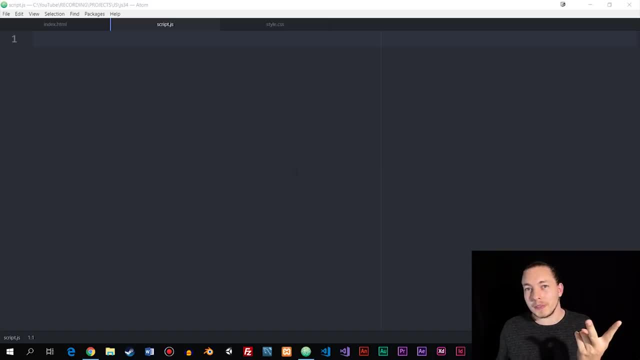 have two types. We have browser-leveled events and then we have DOM-leveled events. Both the browser and the DOM has a ton of different events that you can use And I'm not going to go over all of them this episode because there's way too many to go over in order to explain all of them, But I 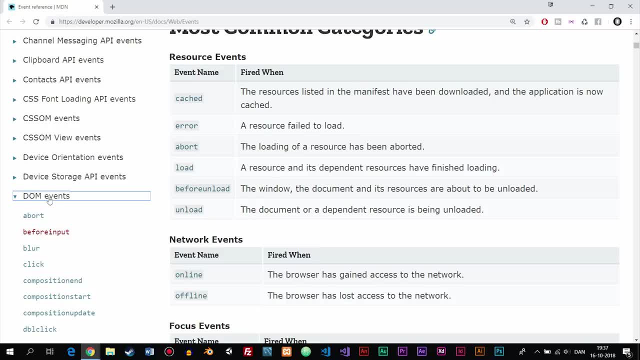 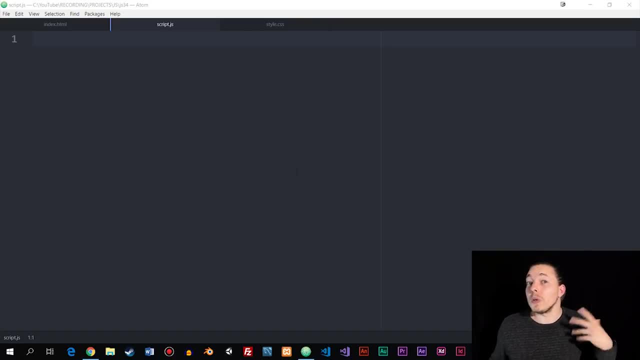 will go ahead and leave a link in the description where you can see a list of all the different events that we have when it comes to browser-leveled events and DOM-leveled events. Now, when it comes to the browser-leveled events, we have something called load, we have something called resize. 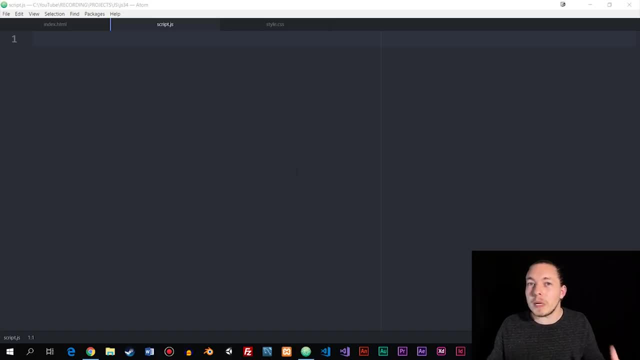 scroll. There's a bunch of different things we can do inside the browser in order to get a website to react in a certain way when we do something inside the browser, When it comes to DOM-leveled events, which is when we do something inside a website. 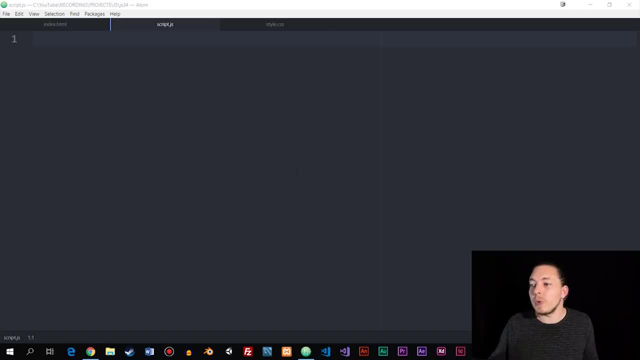 we have a bunch of different ones, such as clicking on something, we can drag our mouse, we can also just move our mouse around- And we also have a bunch of different form-based events which activates anytime we do anything using forms inside our HTML website. So the question is: how do 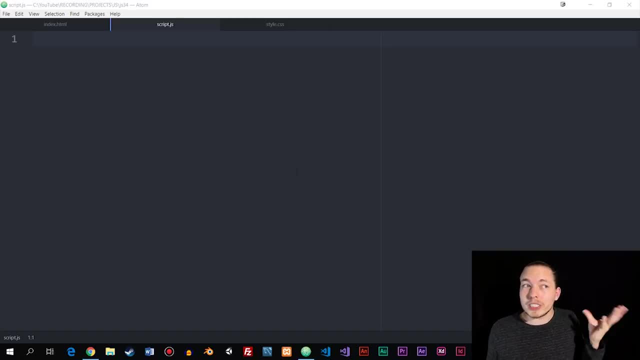 we actually use events inside a website. Well, first of all, we need to actually grab the DOM node or the element that we want to do something with. So we're going to go ahead and do that, And then we're going to do something to in order for something to happen, using JavaScript For. 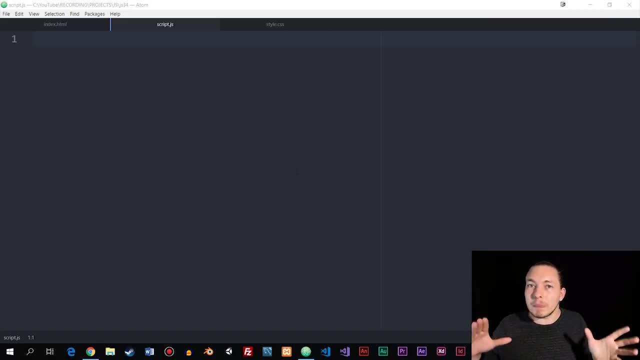 example, if I had a link inside the website that when I click it, then something needs to happen regarding JavaScript. The next thing we need to do is we need to actually tell it. well, now that we have this DOM node, what kind of event do we actually want to happen? Do we want to click it? 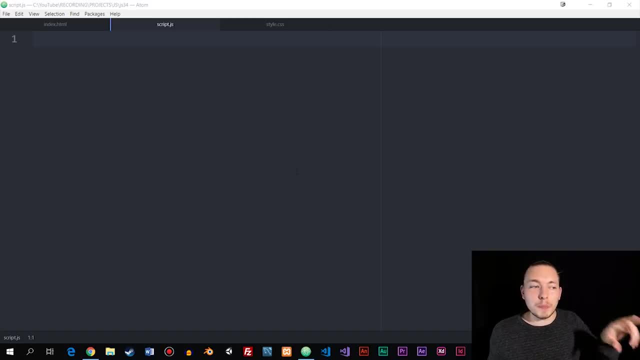 Do we want our mouse to just mouse over it? Do we just want to do something? when the mouse lets go of that specific link, There's a bunch of different events we can apply to that element, And then the last thing we need to do is we need to actually have the JavaScript code, which is, you know, 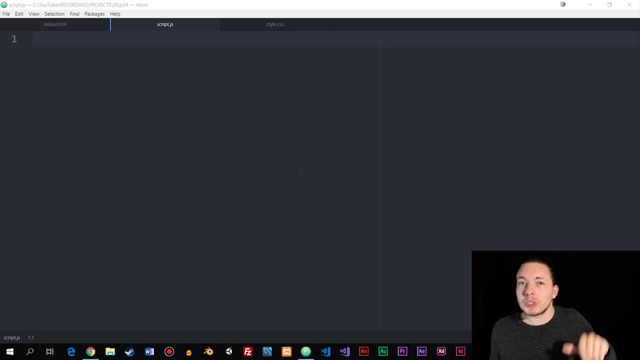 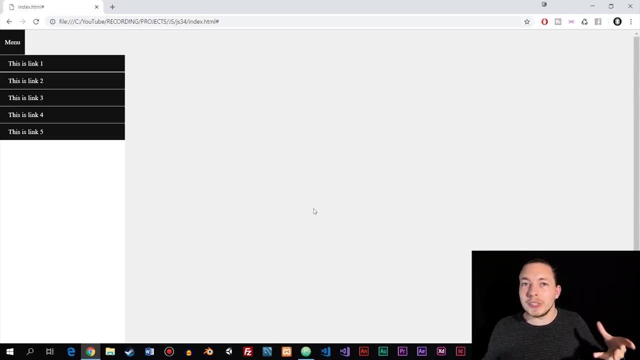 usually a function that needs to run once we do actually do something to that specific DOM node or element. So what I want to do is I want to give you guys an example of how exactly we can use events using JavaScript. As you can see in front of me here, I do have a very basic website. You 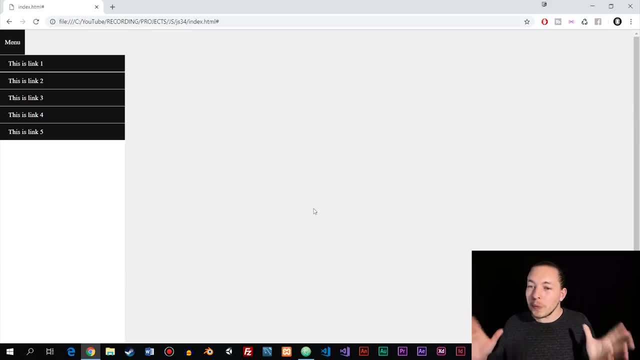 can't really call this a website. It's just a small example, And what I want to do here is I have a button at the top of the website, inside the corner, And once I click that button, I want this specific side menu over here, which has: 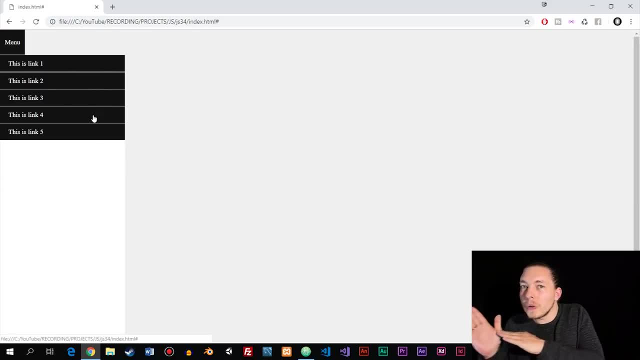 a certain height and a couple of links inside of it. I want it to close to the side or open up from the side when I click that button called menu. I chose this example because I know a lot of you have seen this before inside many different websites. when you toggle, open or close a menu using a 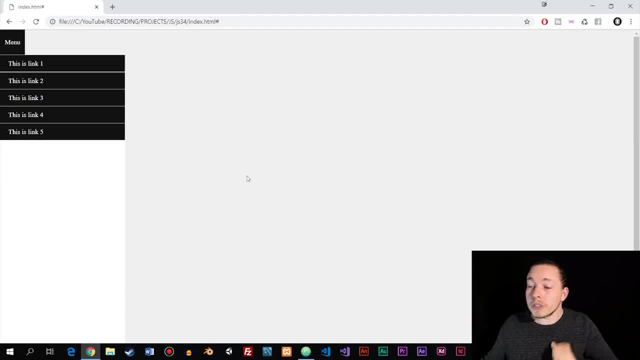 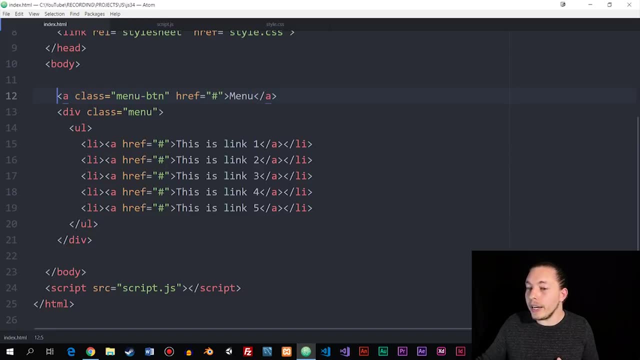 button. So it's something you might be a little bit familiar with. So what I'm going to do is I'm going to go inside my index file just to sort of show you what I have in here Right now. I have a anchor tag that works as the menu button that we click in order to open and close. 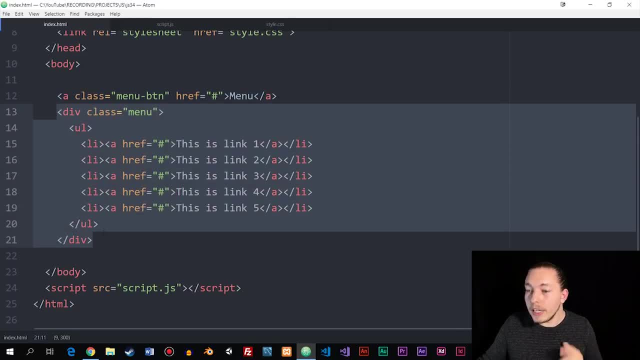 The actual menu, And then I have the actual menu down here. What I did is I just simply start the menu, So we had a 300 pixel width of the menu, And then what I did is: or what I want to do is I want. 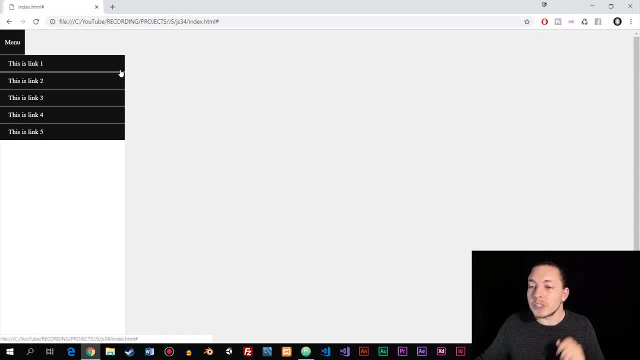 to close this menu when we enter the website for the first time, So when the website loads, I want this to be closed, And the way I'm going to do that is by setting a margin to minus 300 pixels, because then I'm going to push this menu 300 pixels to the left, meaning it's going to go. 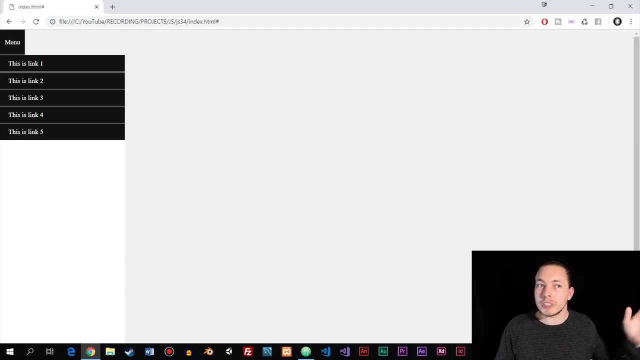 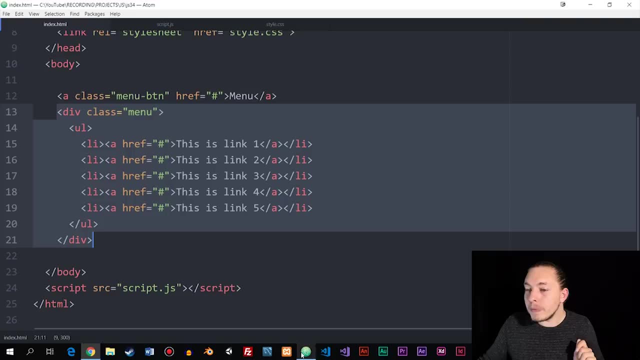 outside the website So we can close it. And then I'm going to close this menu when we enter the website, So we have a zero pixel margin left, meaning that it's just going to jump back in place. So the way we do that is by going inside our script tag. And the very first thing I want 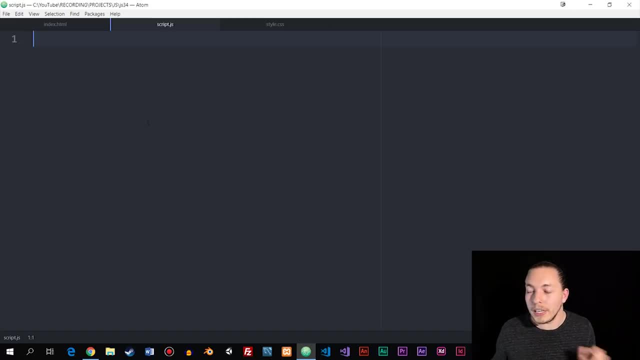 to do is I actually want to grab the elements that I'm going to do something with. So first of all, I'm going to say we have a let type variable And I'm going to go ahead and call this one menu button So menu BTN- Let's actually spell that correctly BTN- And I'm just going to go ahead. 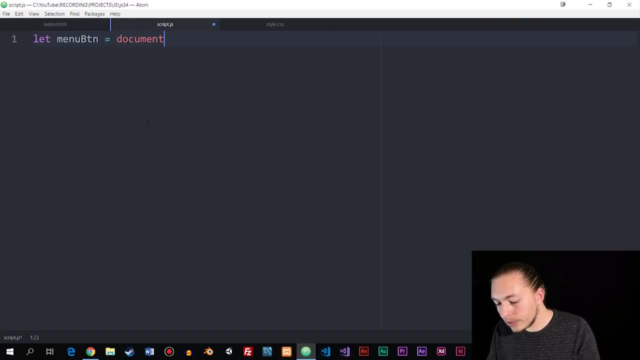 and say, menu is equal to documentquery selector- parentheses. And then I want to select, first of all, the button that we're going to click on, which is going to be the one that we attached the event to. So when we do something, this button here. something needs to happen, So I'm just going. 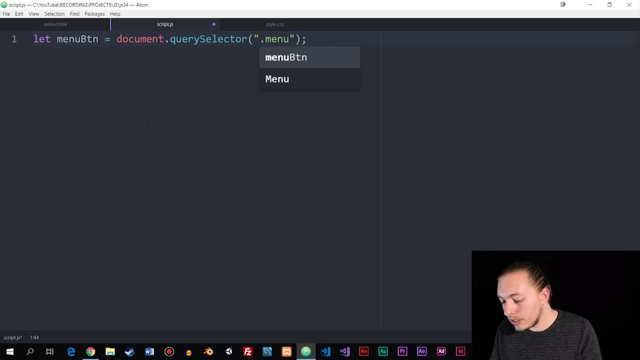 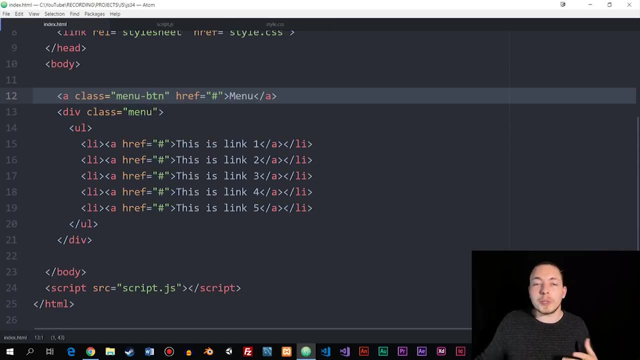 to go ahead and refer to a class I have called menu- button which, again, if I were to go inside my index page, as you can see is right here. The next thing I want to do is I want to say menu. 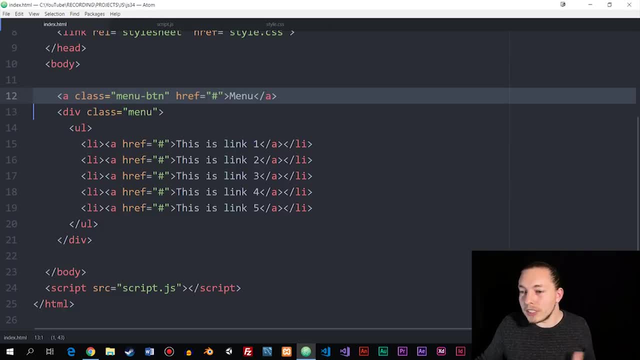 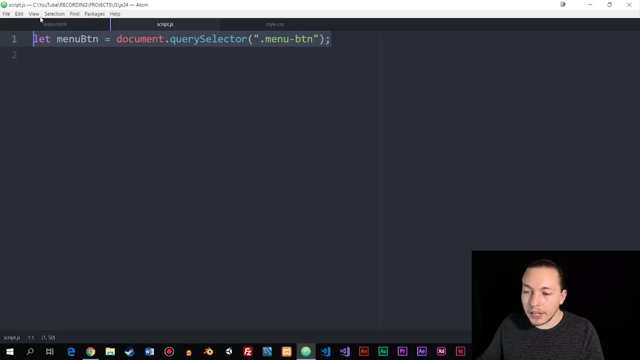 to grab the actual menu that i want to do something to. so, as you can see, i have a class attached to it called menu. so i'm just going to go back inside my script tag or inside my script file. i'm just going to go ahead and copy paste this line of code and paste it below here, then i'm going to call it. 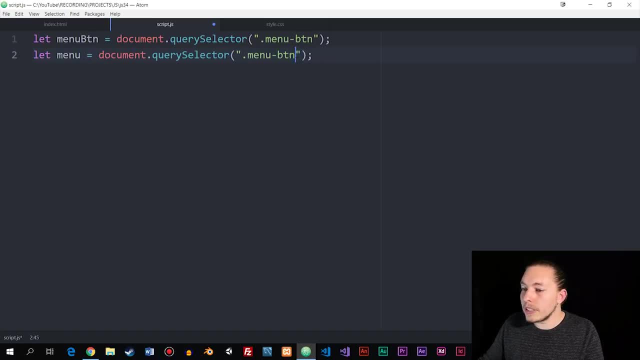 something else like menu, and then i'm just going to go ahead and change the class name in here to menu. now the next thing i want to do is something that we do quite often inside javascript. now, we could have done this differently. we could have applied a class to this div element, that is. 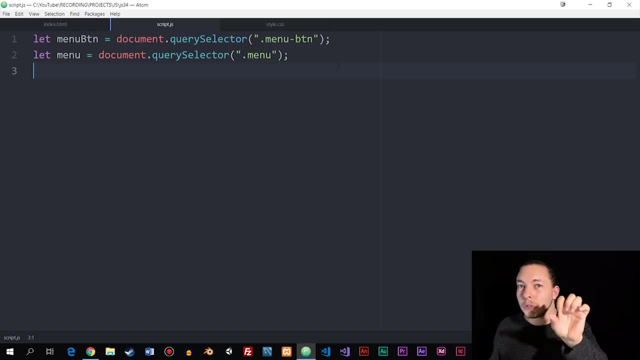 sliding in and out, where we just apply the class in order to give it a zero margin and then we remove the class in order to push it back in. but i decided to do it in this way, where we just simply change the css, because it's something we've done a lot of before in some of the previous lessons. so 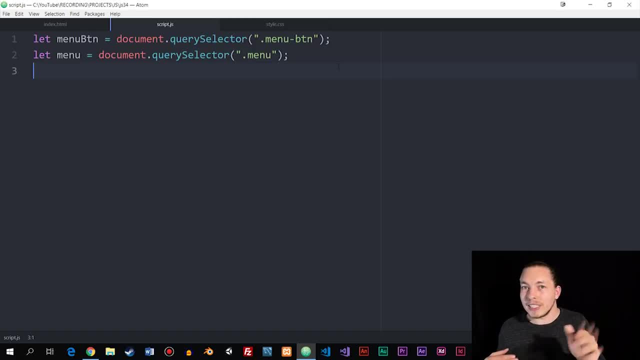 that's why i chose to do in that specific method in this episode, just in case anyone is wondering. so what i want to do is i want to have a sort of status that tells me is this menu open or is it closed. so what i want to do is i want to create another. 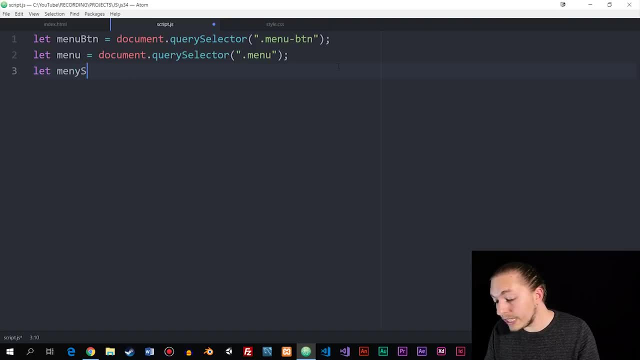 variable. i'm going to call this one menu toggle or menu status would actually be better, like so, and again i spelled menu wrong. i have a habit of doing that. so status, and i'm going to set this one equal to false because i want it to be closed once we go into the website. 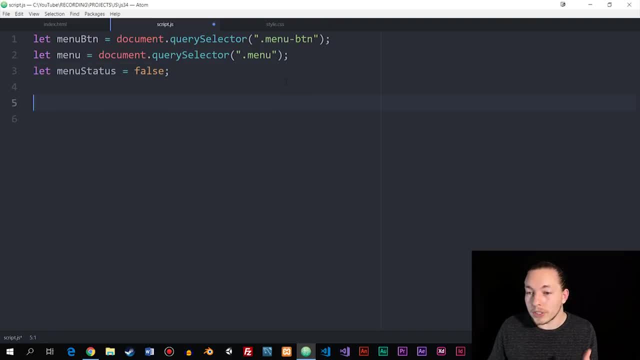 so what i want to do next is i want to actually create the function that is actually going to toggle it back, open and close it. so i'm going to create a function here. so i'm going to say function, i'm going to call this one menu toggle. 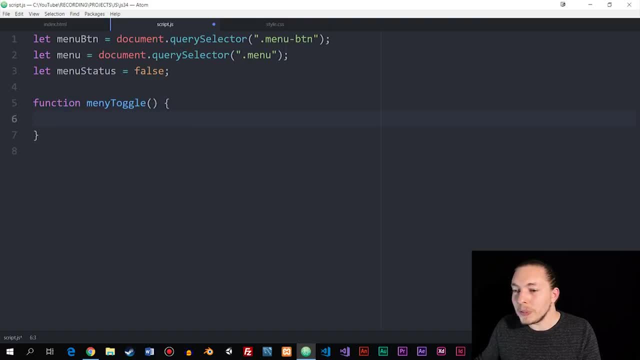 parentheses, curly brackets. and again, i spelled menu wrong. i have no idea why i keep spelling that in that way. it might be because in denmark we spell it with a y at the end, so that's why i keep making the mistake. um, so, inside the function here, what i want to do is i want to run an if. 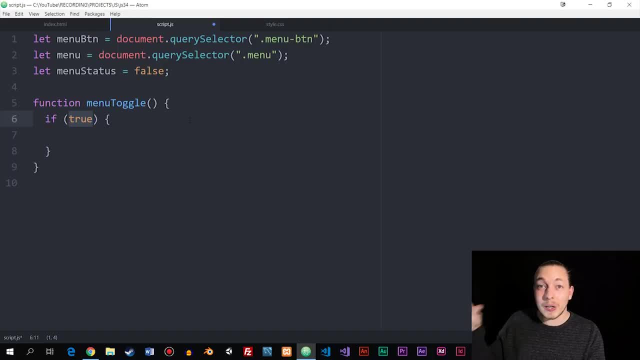 statement because i need to check: do we actually have the menu open or is it closed? so what i want to do is i want to say: well, is menu status equal to false? if it is equal to false, then we need to open it inside the website. then. 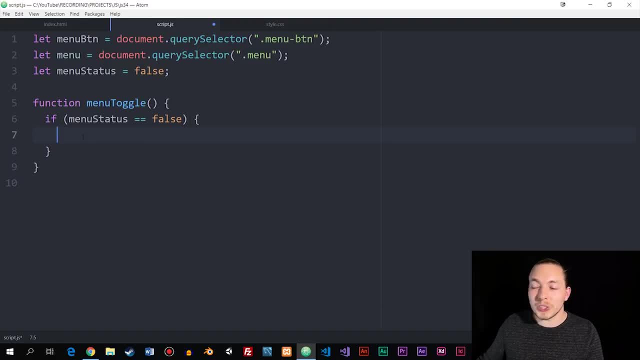 what i want to do is i want to grab the menu from up here that i want to do something to, and then i want to apply a styling to it using javascript, so we're going to use the style property, and then i'm going to say i want to style the margin left and then i want to set it equal to. 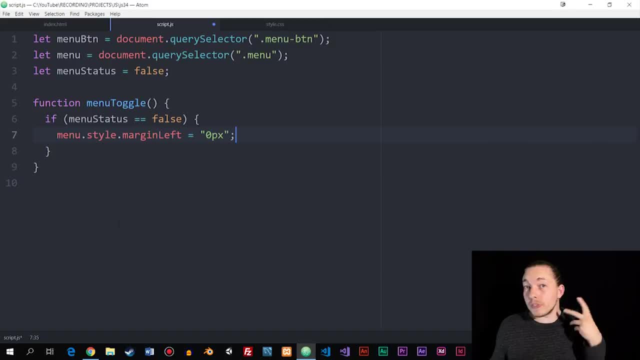 zero pixels, because right now, if we have a menu that is false, then it's going to be closed. so i want to open it up, so i want to disable the negative margin by sending it to zero. then what i want to do next is i want to change the menu status, which is up here, from false to true. 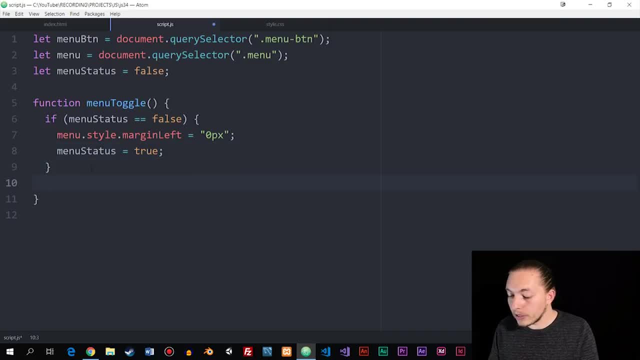 next thing we do is we go down here and create another. uh, we can create an else if statement, so we can say else if. and then inside the else if statement, we want to do the opposite. so instead of taking for a false statement, then we want to check for a true statement, and then we just copy paste. 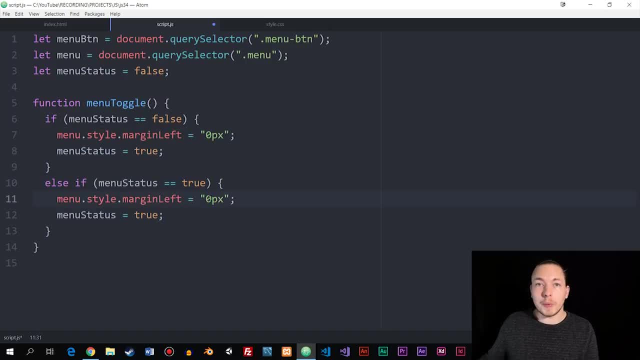 have here and do almost the exact same thing, except this time we want to revert it back to negative 300 pixels with the margin. so i'm going to say negative 300 pixels and then we want to change it from true to fault so that next time i click the button it's going to go back up to the 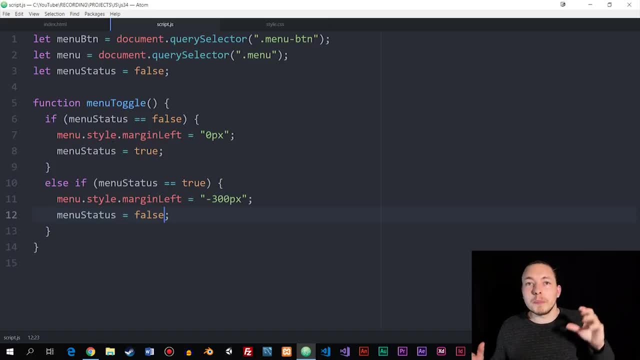 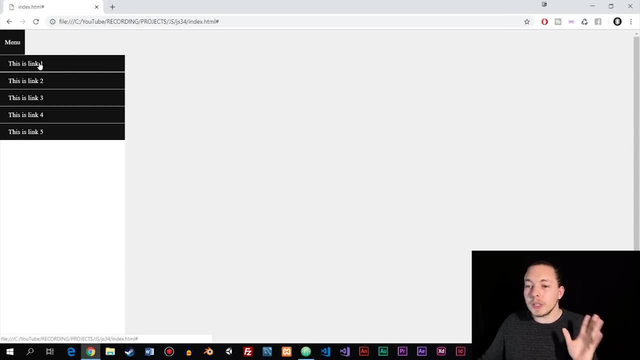 first if statement up here. the next thing i need to do is i want to make sure that the menu is actually closed once we load up the website, because if i were to go inside of it inside the browser, as you can see, once i refresh, it is still open inside the browser. so what i want to do? 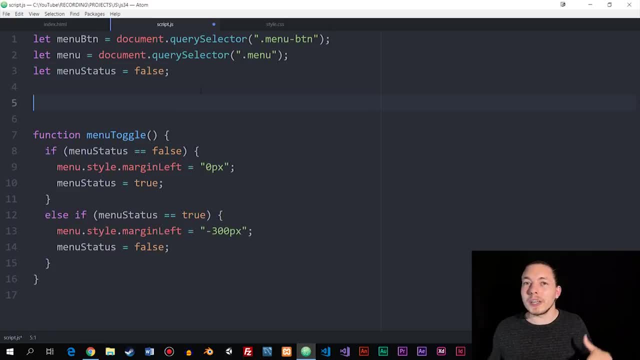 is right before we have the function, and what i want to do here is i want to run a little bit of javascript code as soon as the website is loaded. so what i'm going to do is i'm going to apply a little bit of styling to the menu, so i'm just going to go ahead and copy what we have down here. 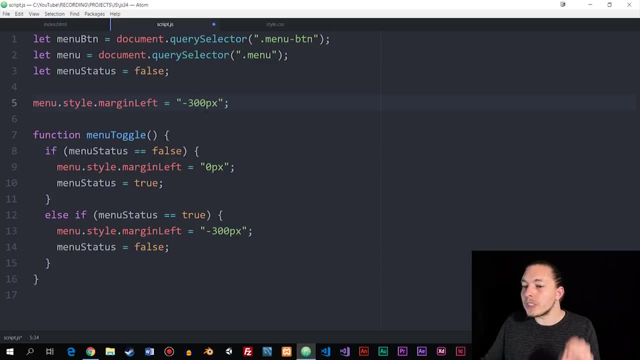 inside the else if statement. i'm just going to go and paste it up here because as soon as the website loads, i want to start with a margin set to 0 negative 300 pixels. now you could argue that you could go and start the style sheet and just go ahead and apply a negative 300 pixel inside the styling. 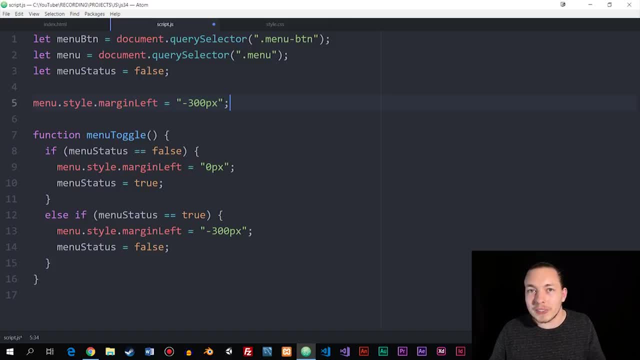 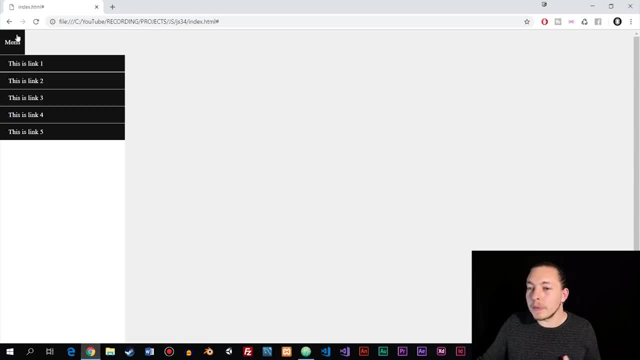 and you could do that. i mean, it's up to you, but i just want to do it using javascript, because this is a javascript lesson, so why not do it in that specific way? so i'm going to just go ahead and save it here. then i'm going to refresh the browser and, as you can see, we now have a closed menu, the. 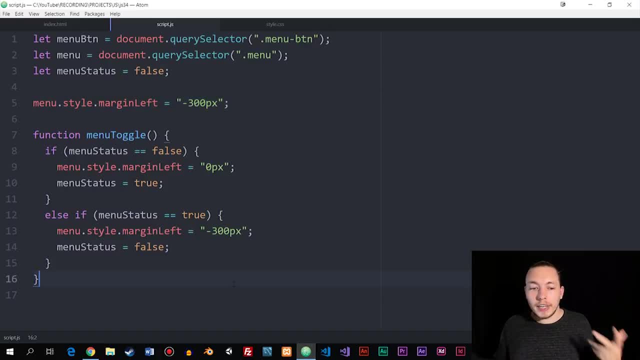 next thing we need to do is we need to create something called a event handler. now, what an event handler is is actually that line of code that goes into the website and says: once we do something to this specific dom node, then run this piece of javascript code, for example, a function. 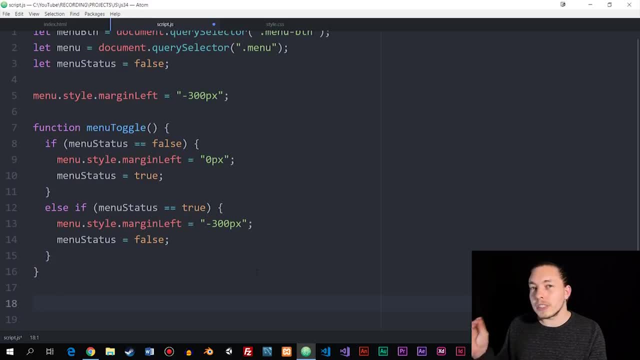 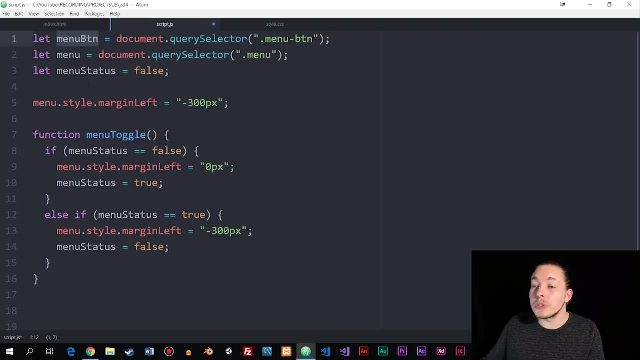 so what i'm going to do at the bottom here is i'm going to say, well, when something happens to one of the dom nodes, i'll need to actually grab that specific dom node. in this case, i did actually refer to the menu button up here. i'm just going to go ahead and copy it, paste it below here and 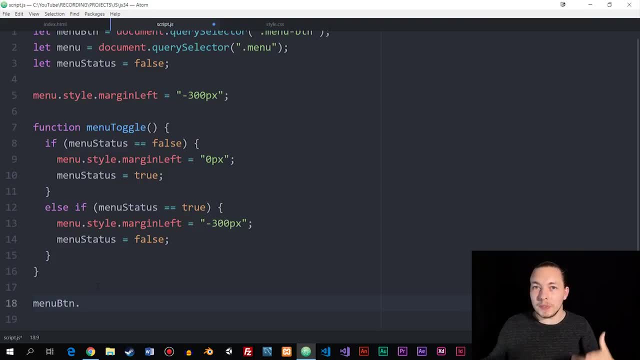 then i want to say: what kind of event do i want to happen to this specific object? and in this case, here we could just go ahead and say we want a on click event, which is a very typical one to have when you want to click on something and then something happens. 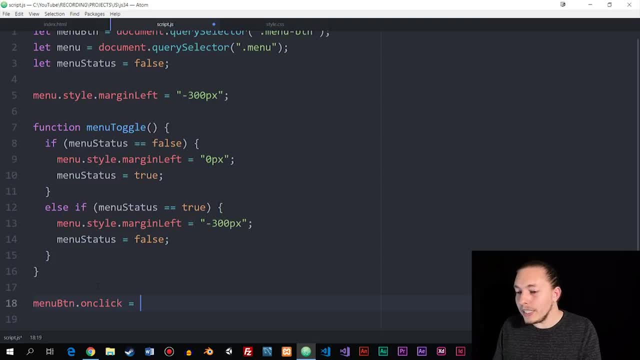 so we can't just say on click, and then i want to set it equal to the specific function i want to run once we actually click this specific object. now i do want to point out: when we do actually refer to a function like the one i have up here called menu toggle, then we don't add the 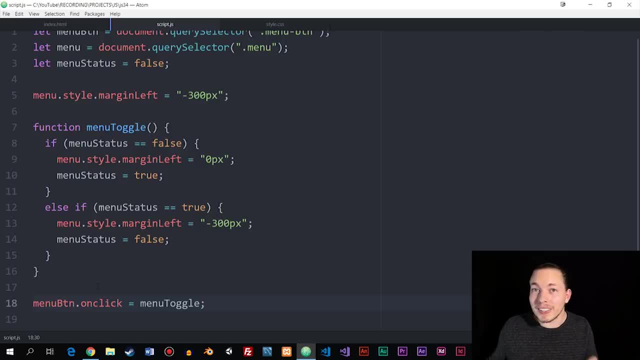 parentheses at the end. otherwise this function is going to run once the code actually gets loaded. so in order for the function not to get run immediately once we load up the function, we can't actually have the parentheses at the end of the website. we need to not have the parentheses behind. 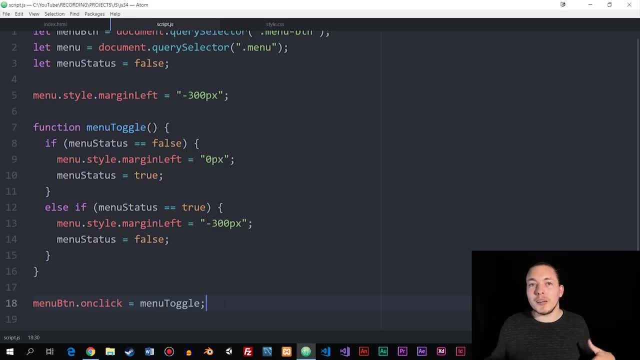 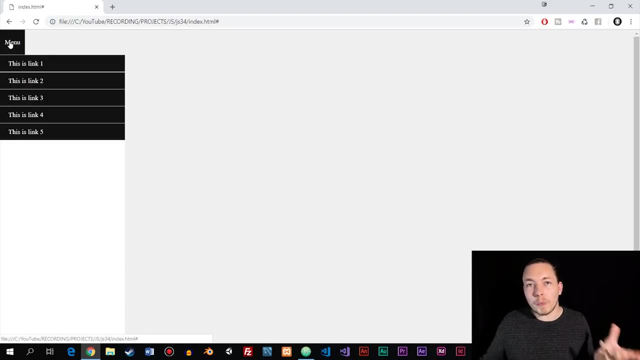 here. so that's a very important detail. so once we do this, we do actually have a event handler. if i were to go inside the website, refresh the browser, click the button. you can now see that we have a open menu inside our browser. if we were to click the button again, you can now see that we close. 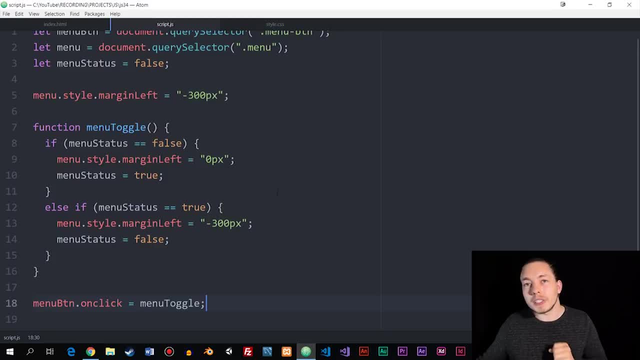 back down the menu. now i do want to show you one more thing, which is a typical thing i see people do when they use events inside their html. when it comes to using javascript, in fact, go inside your. if you were to go inside any of your html files and go inside one of the 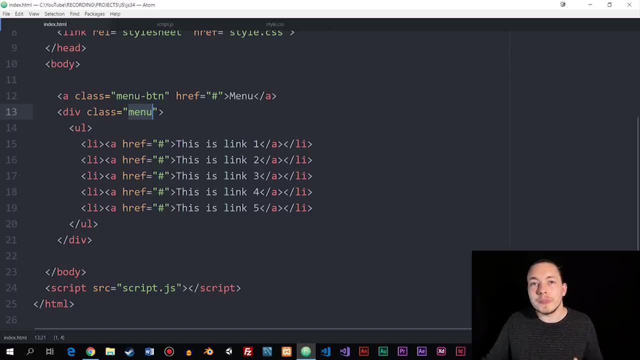 elements inside one of the starting tags, you can actually go and apply events directly inside the html. so if i want to go inside this specific div tag here- actually let's go ahead and take the, the anchor tag we have up here- i can go ahead and write an attribute with the name of the event. i 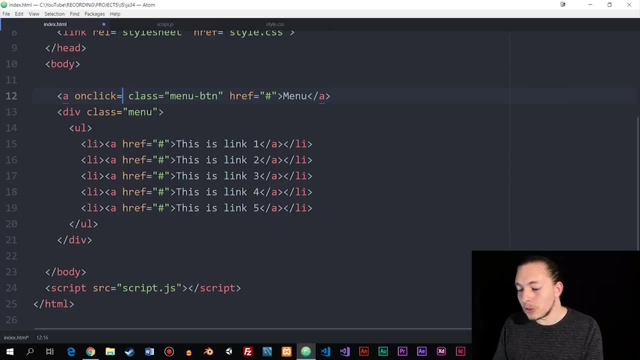 want to run, so, for example, on click, then i want to set it equal to the function that i want to run inside this specific element here, so i could actually say menu toggle and, as you can see, when we do actually add events in line with the html, then 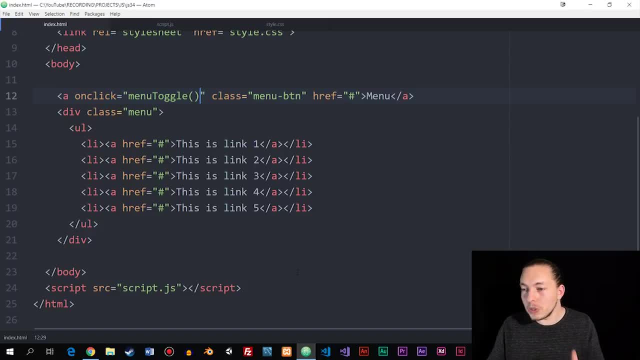 we don't need to neglect the parentheses at the end, so we do need to include them here in order for it to know they want to run a javascript function. so this is how we do events inside javascript. so in the next episode i'm going to show how to prevent some default events from 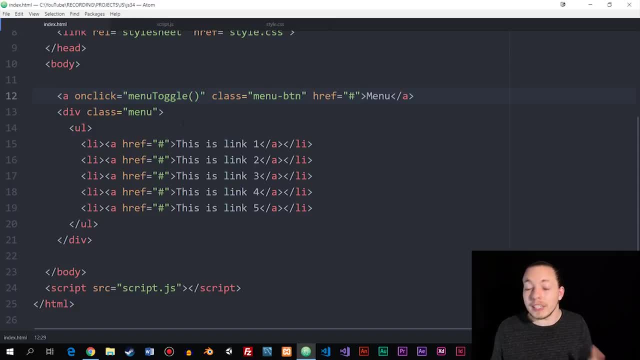 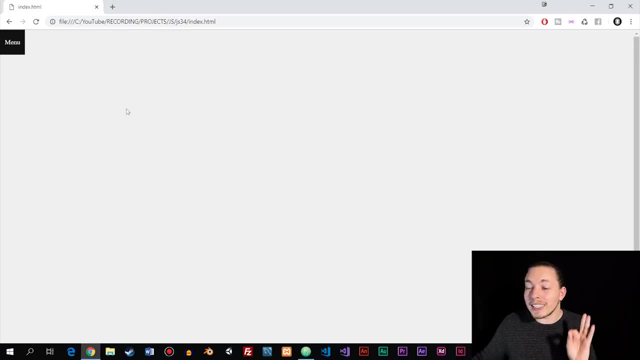 happening on some different dom nodes that you have inside your website. now, just to show you what i mean when i say default events, let me actually go and go inside the browser now. i want to refresh the browser here when i click this button up here, which is technically a anchor tag. 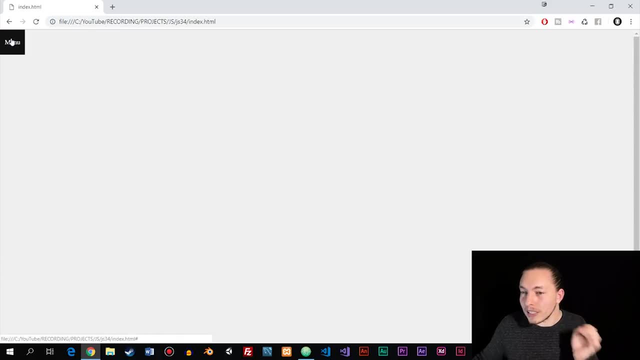 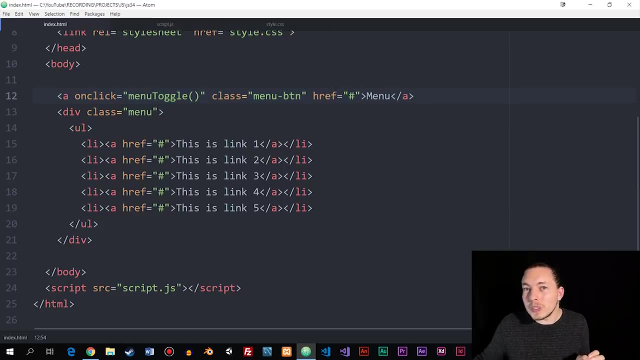 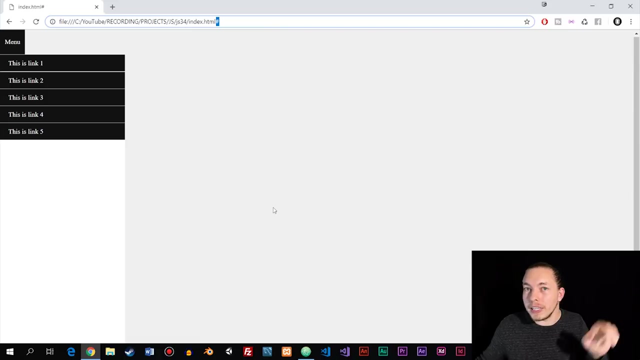 inside the html. you'll notice that inside the url, when i click it, we get this little hashtag symbol because it's not linking to anywhere inside our website and when we do this, the website is going to refresh the entire page, meaning that if i were to have been scrolling down on the page and i 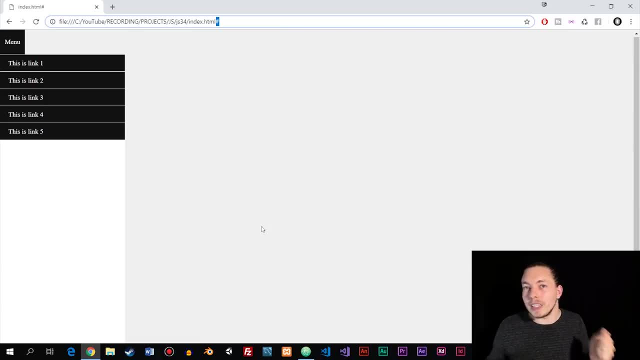 were down at the bottom of the website and then i want to fire up some kind of javascript event, then it's going to take us back up to the top of the page, which might not be an effect we want to have in some cases with forms as well. if i want to, 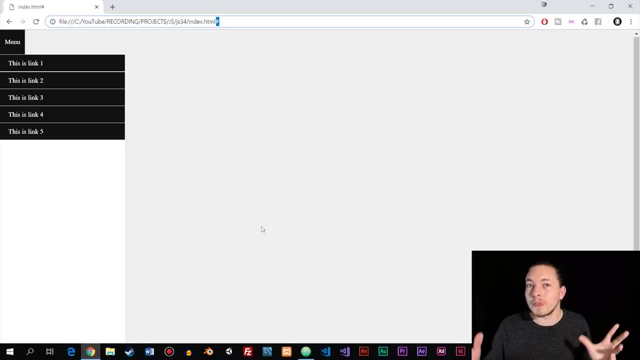 not submit a form directly, but i want something to happen using javascript before we submit the form. then we also need to prevent the default event from happening in some of these elements. so that's what i'm going to teach in the next episode. so i hope you enjoyed and i'll see you in the next. episode so.